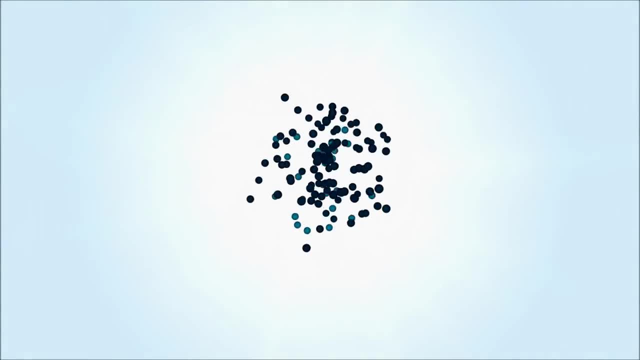 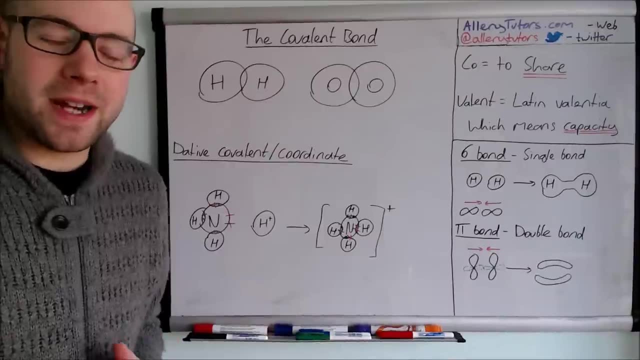 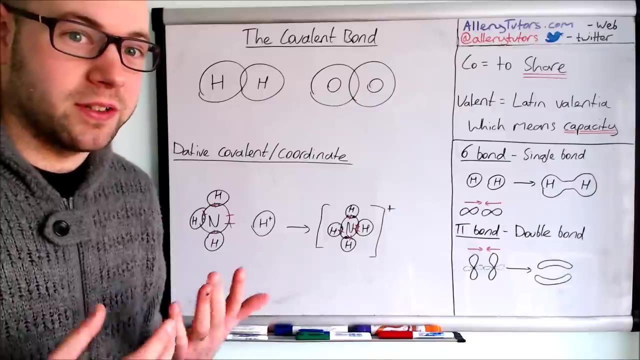 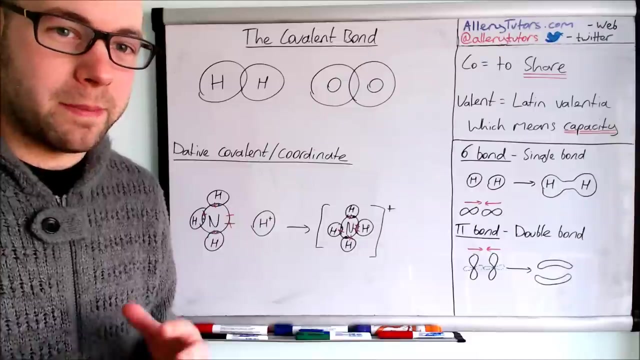 Hi there, my name is Chris Harris and I'm from AlleryTutorscom, and welcome to this video on the covalent bond. In this video, we're obviously going to look at the covalent bond. we're going to look at dative, covalent and coordinate bonding as well, and we're also going to look at some a bit of. 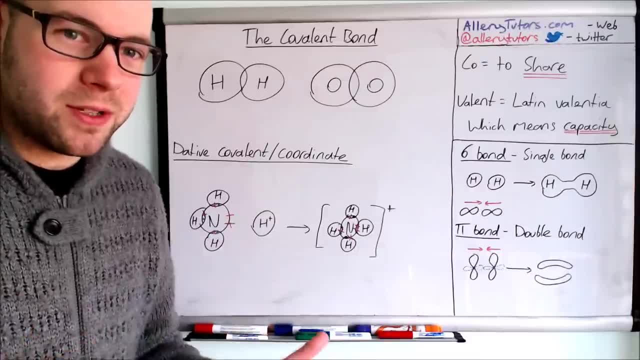 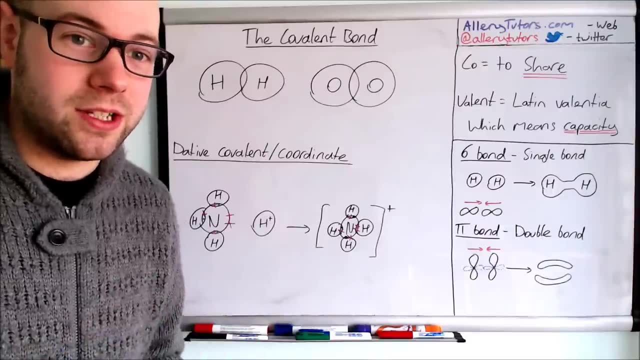 orbital stuff as well. So you might be thinking: well, why do I need to watch this video? I don't know what covalent bond is, I've done it at GCSE- but in this video we're also going to look at some additional stuff that you need to know for A-level as well, and some of it can be actually quite 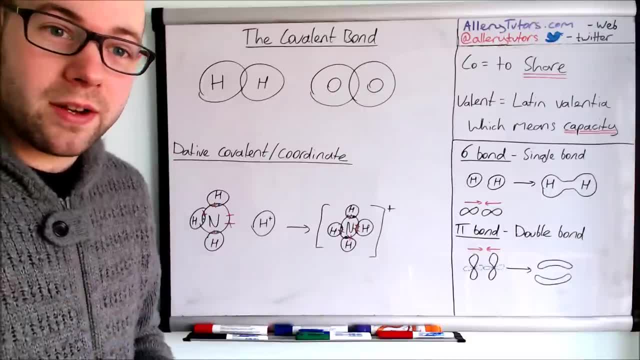 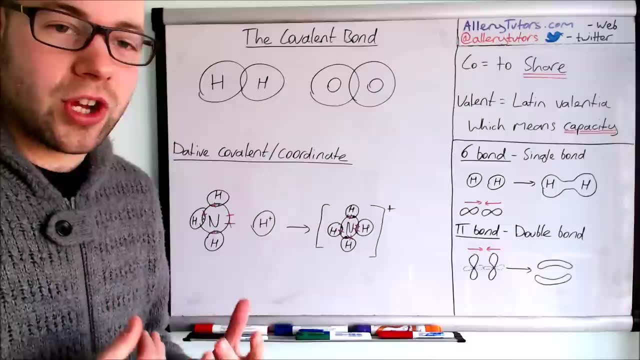 tricky and they look very abstract. so just tune in for about another five or six minutes to make sure that you know everything you need to know about the covalent bond. Okay, covalent bond, co means to share, and valent actually comes from the word valentia, which means capacity in Latin. 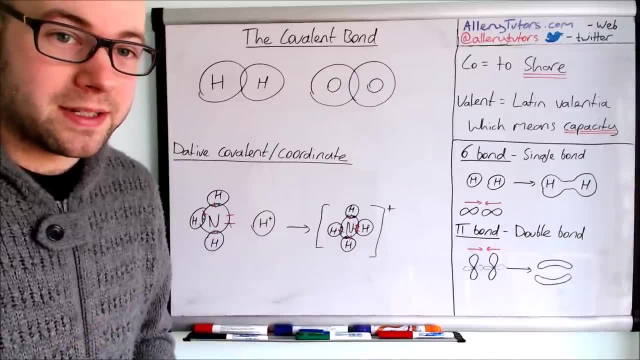 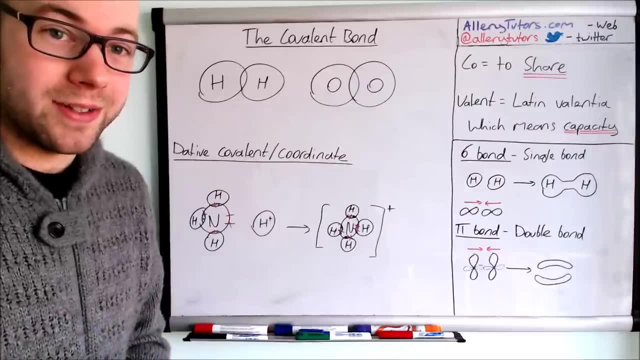 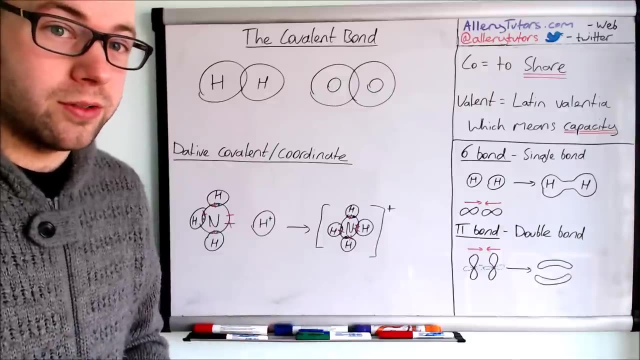 So if we put them together, it's basically the capacity to share electrons. in other words, how many electrons can an atom share? Now, according to the basic laws of chemistry, the first shell can only hold two electrons, and then the shells after that can hold eight. Some shells can hold 18, depending if they have d orbitals as well, and 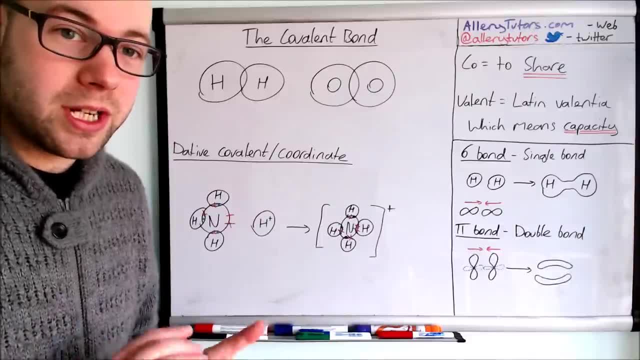 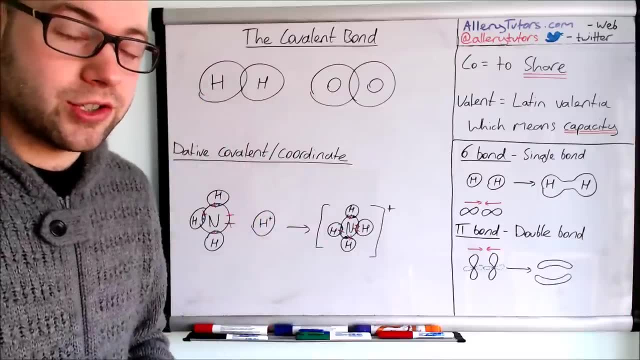 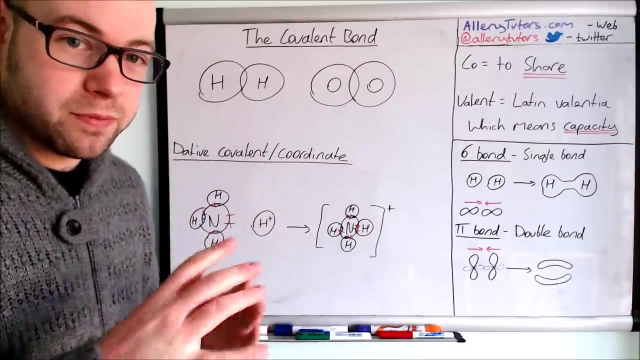 some can only more if they have f orbitals as well. but we're just going to keep with the simple principles here for the time being. So you can see, here we've got a hydrogen atom, we have the outer shell and we're going to show how the kilobytes are going to form a solid cell. So the basic. 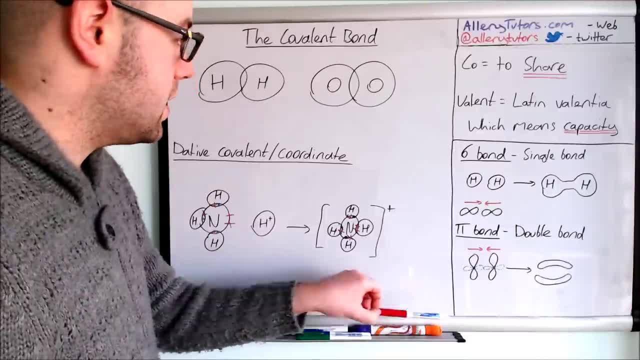 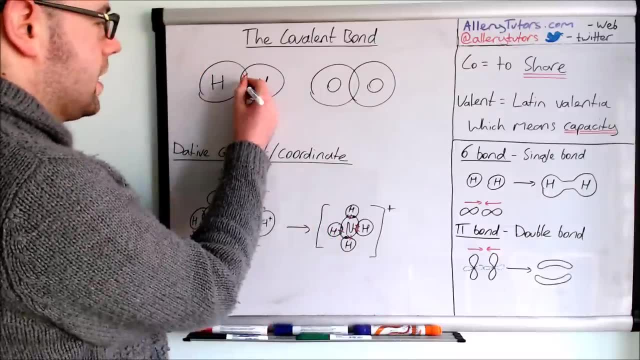 principle is basically they share electrons to form two electrons. So they both have two electrons in the outer shell for them to become stable. So we're going to add the electrons in here. So you can see, one hydrogen will have one electron there and the other hydrogen will share the other one. 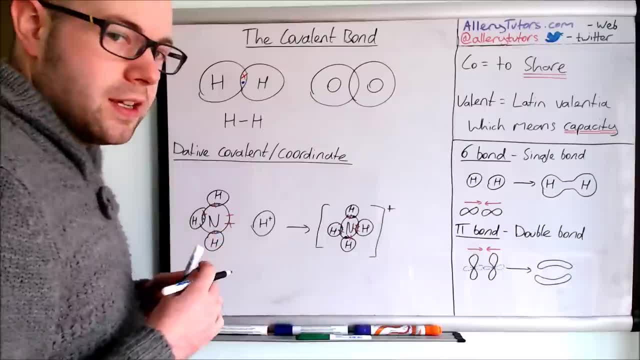 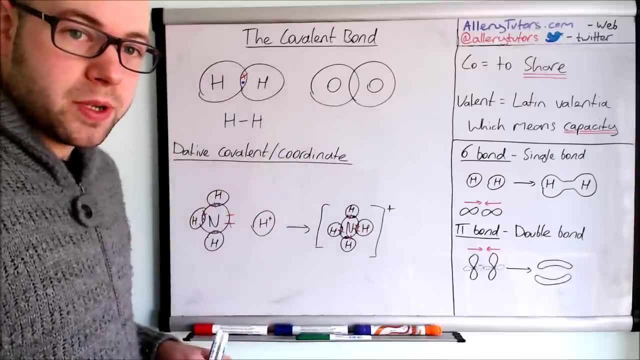 like that, and the basic idea is that when we draw our molecule, we draw it with a solid line and that shows a covalent bond. So that's pretty straightforward- Something you would have done at GCSE- to form a double bond or maybe a triple bond, and so in this case, oxygen has six. 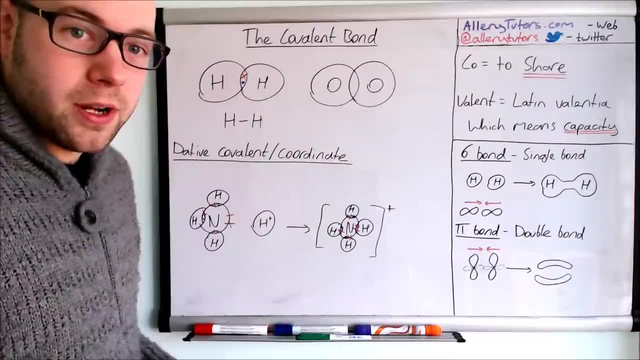 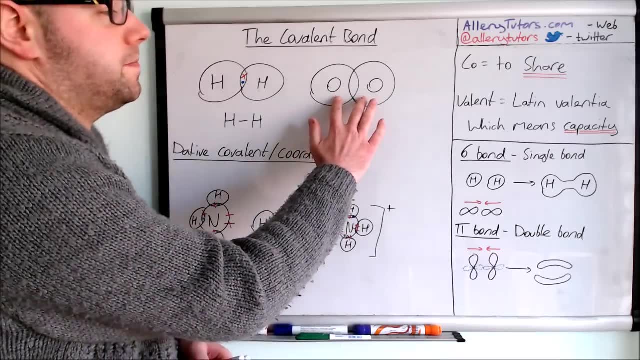 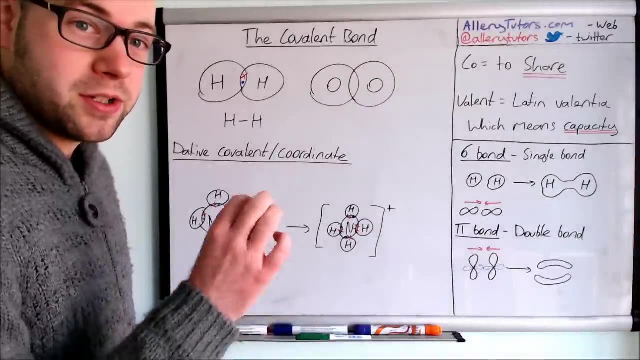 electrons in its outer shell. it needs two electrons to become more energetically stable, and so therefore it needs to share two electrons, and and for each atom. so remember, the sharing of electrons is, the sharing of pair of electrons is for current bonds. make sure you get the word pair in as well. so 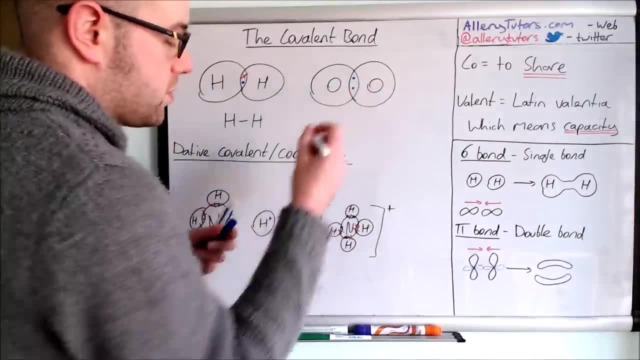 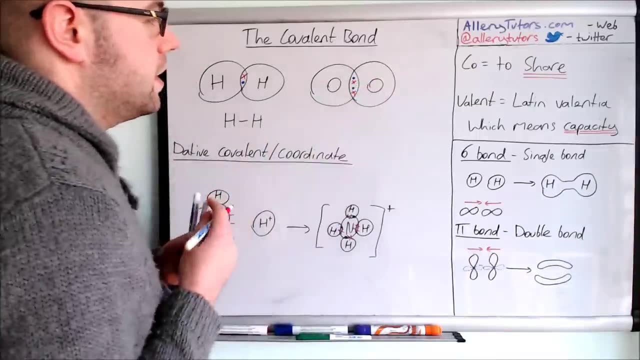 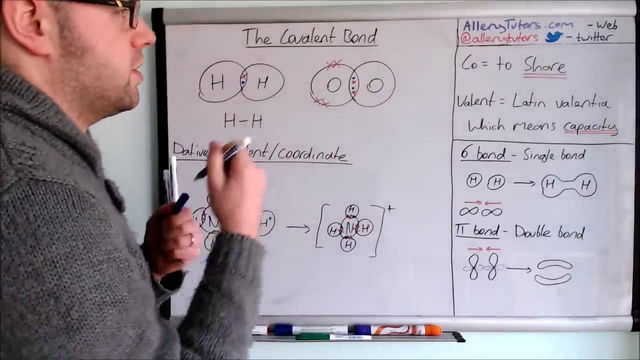 let's put our electrons in here, so we've got the blue ones will represent one oxygen atom. we're going to put them as a dot and the crosses represent the electrons of the other oxygen atom. now oxygen has six electrons in total, so let's put our other electrons on there as well to make sure that we're being 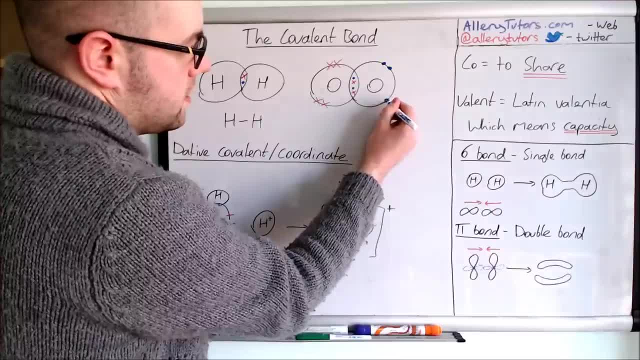 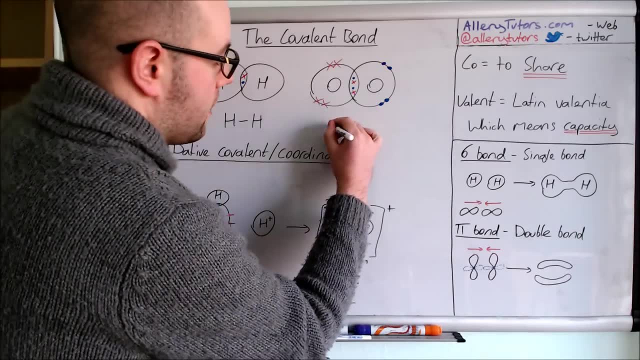 very, very clear. they can see here that by doing this you can see both oxygens now have a full shell of electrons, which makes them energetically stable, and we can draw it like this double bond oxygen. so, yeah, pretty straightforward. so this is something that you would do. 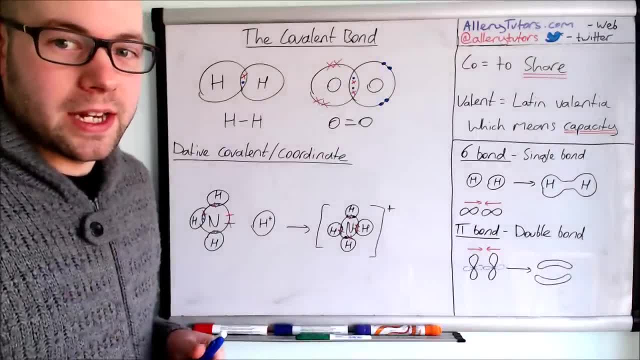 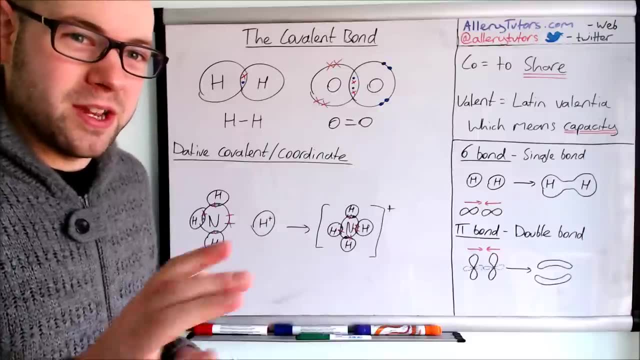 a, a, a, a, the electron orbitals over there at GCSE level. let's go into the a level bit. then let's extend it that little bit further. the single bond now has a new name for a level chemistry in particular. it's not quite new, it's actually been. 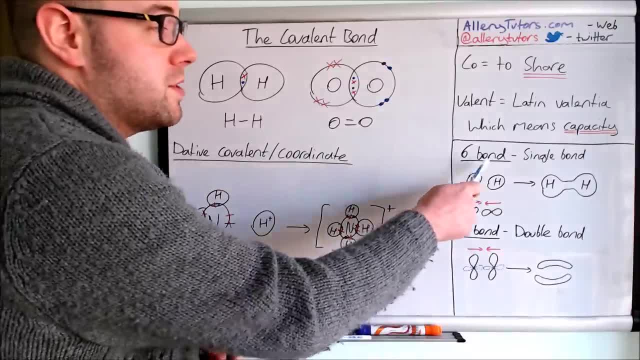 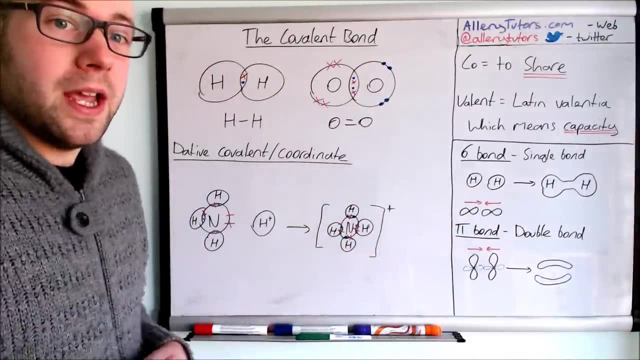 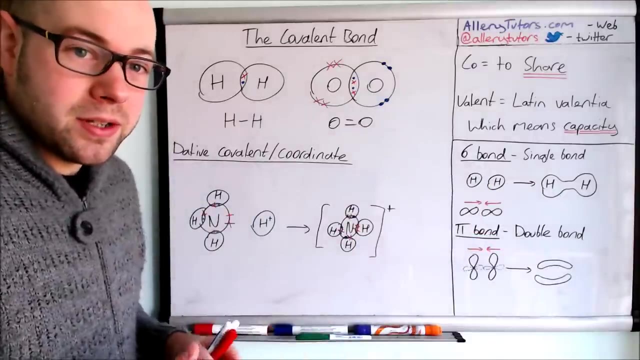 out for years and years. but in terms of your content and you need to know, the single bond is a Sigma bond and a Sigma bond is basically where the orbitals will overlap each other and and we form this looks a bit like a dumbbell and this is effectively a Sigma bond. so when the electron orbitals over there, 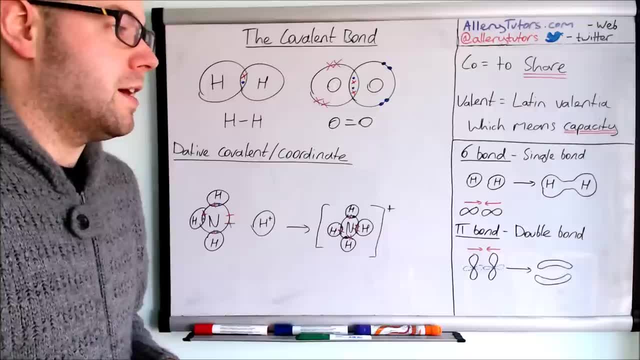 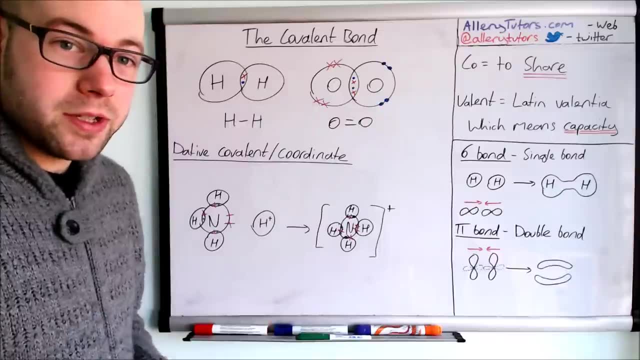 and there are a pair of some number of shining of electrons and there's a pair of electrons in the middle, and so that is the covalent bond. now that would be the case of it is an s orbital. if we have p orbitals, a Sigma bond is where two. 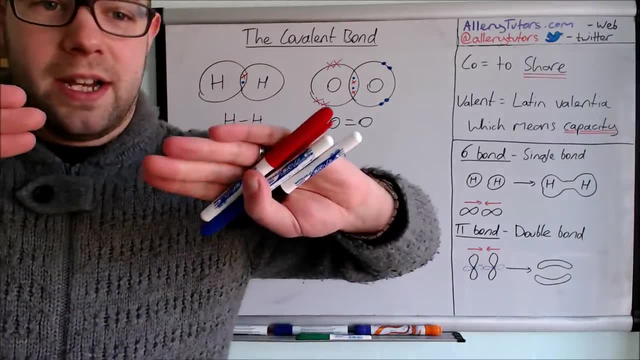 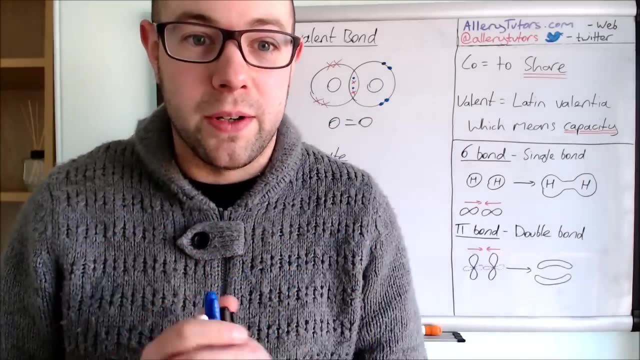 P orbitals like this but actually come head to head, so the kind of approach a little bit like this and they would squash together like that and not overlap. there is the actual bond that's been formed now when you've got p orbitals over up and head to head. we call it a covalent bond like that and we've got a. 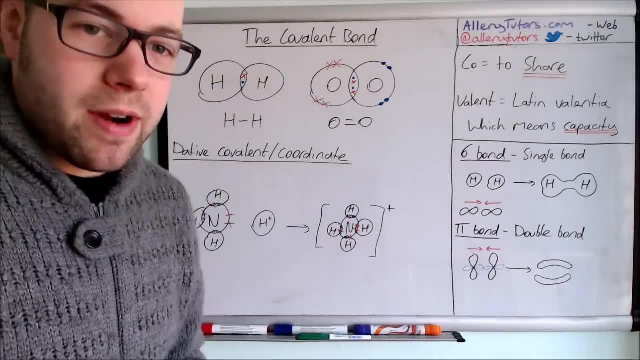 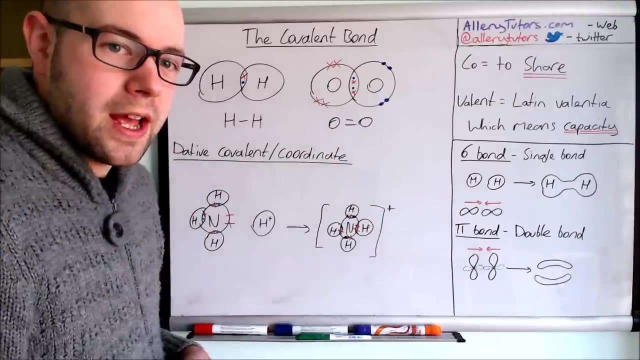 We call that a sigma bond, And so that's what we've represented there. Now, the sigma bond. obviously each one of these has the electron in there and it will then overlap and it will share And that's your covalent bonds. So quite strong- actually reasonably strong- bonds and covalent bonds. 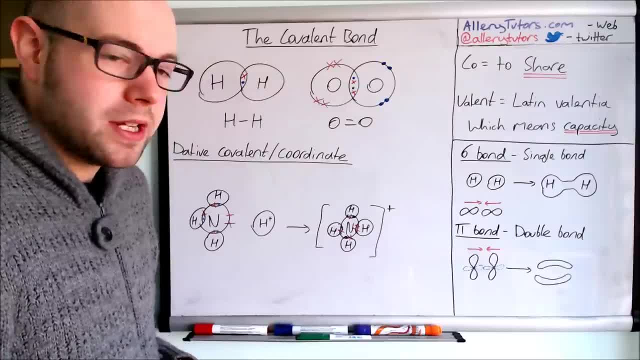 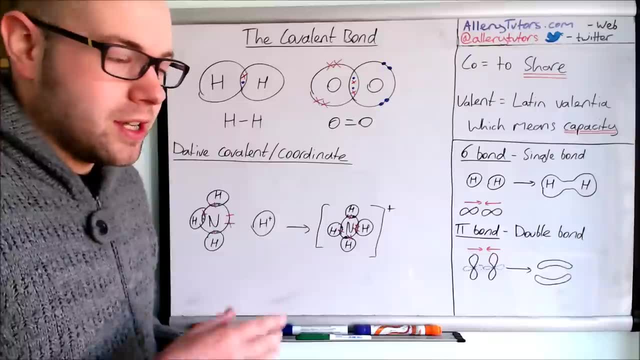 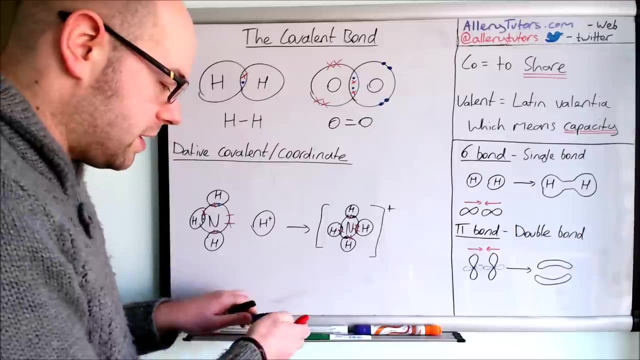 And the other type of bond, though, is a pi bond. Now, pi bond is also known as a double bond, And it's not quite strictly true, as I'll show you in a minute. A pi bond is actually when we get, say, for example, we have p orbitals here, when p orbitals actually come together, but they're actually approaching side by side. 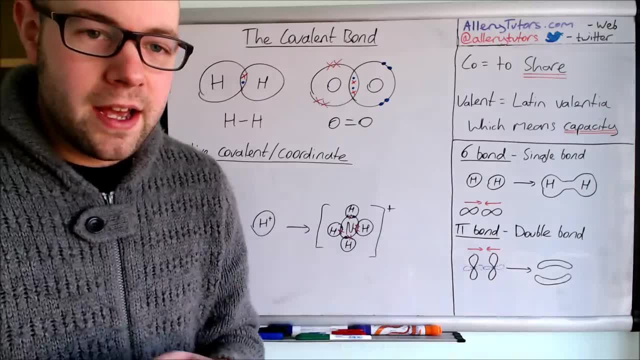 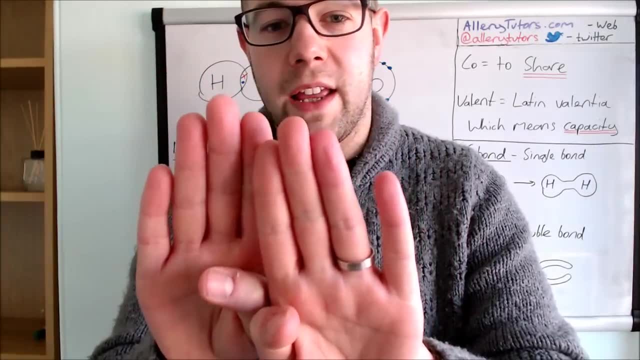 So you might have the lobes of the p orbital, as you can see here, and they're coming together, but they're approaching from like a side view, like this. So if I stand in front of the camera and they actually approach like that, so you get a much bigger overlap compared to just like that. 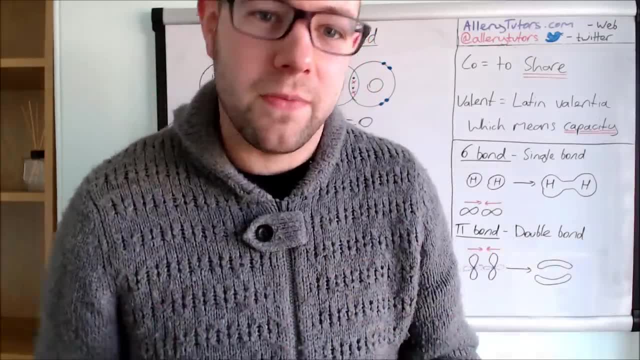 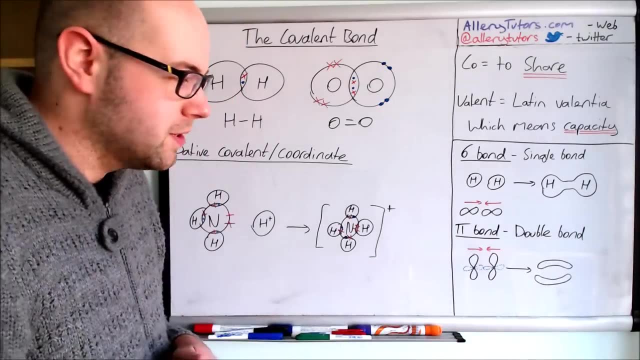 So that bigger overlap effectively gives you that extra strength. what you would find in a double bond- And you can see here what I've also done is I've drawn in blue like a dotted line looks like a ghost orbital- is effectively the pi bond here, the sigma bond, sorry that we had before. 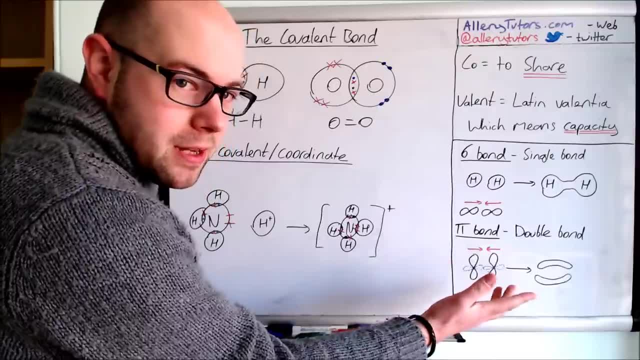 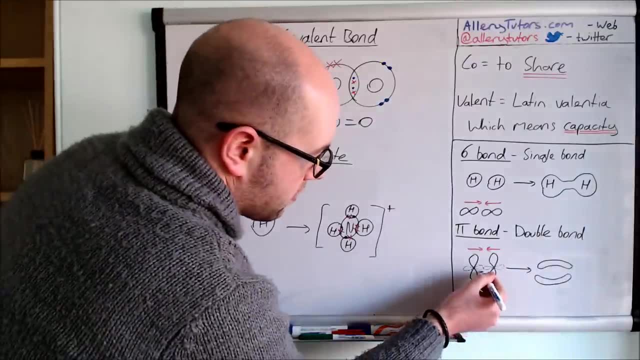 So there's the sigma bond. You can see the orbital in the same atom, exactly the same atom. These merge together and this would form the sigma bond there. So I'll just add that in. That's just to show where the sigma bond would fit in. 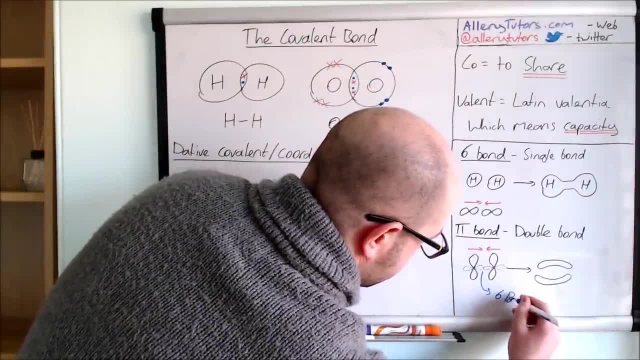 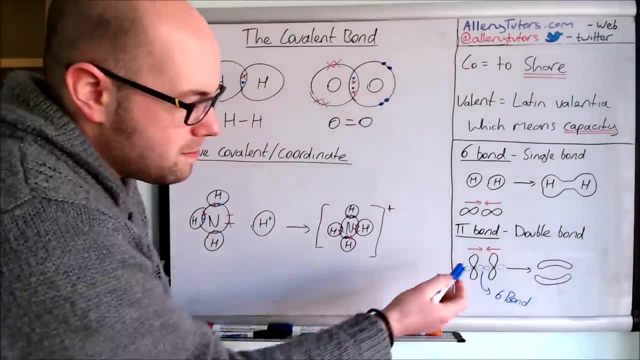 So we'll put that in there. So that's the sigma bond in the blue And in the black. these two would. Now you can see it forms this funny shape because in the middle of the orbital it actually nips in at the middle and effectively it's like a figure of eight. 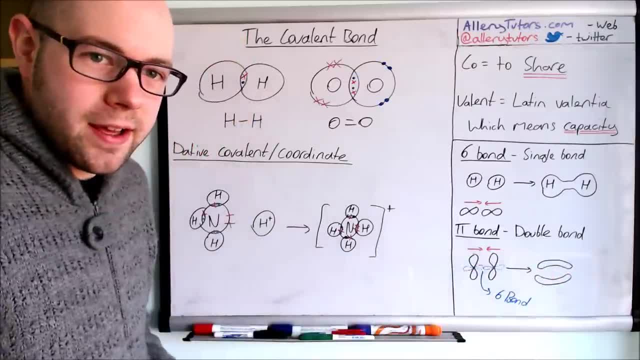 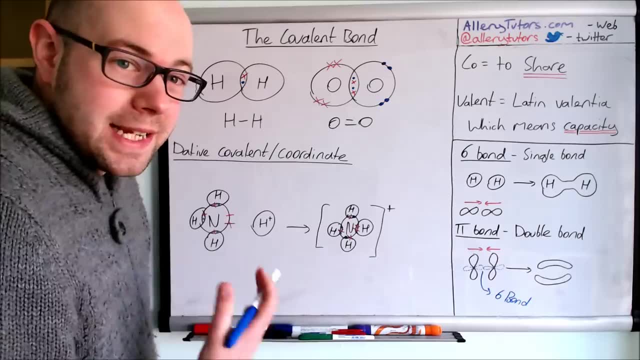 So when we merge these two together, we actually end up like this: It looks like a like a hot dog bun with a hot dog in the middle of it. So this, these are your sigma bonds, And this is obviously quite a strong bond. 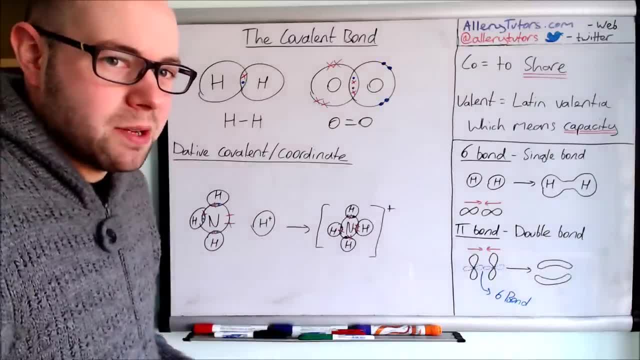 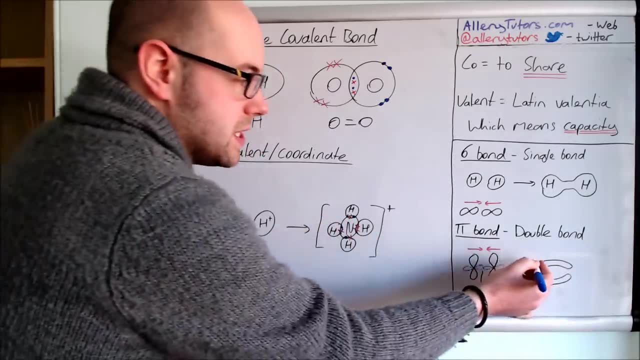 Now the reason why I didn't say this was strictly a sigma bond is actually when you have a pi bond- Sorry. Why This isn't Strictly a double bond is because this pi bond here actually will contain a sigma bond as well. 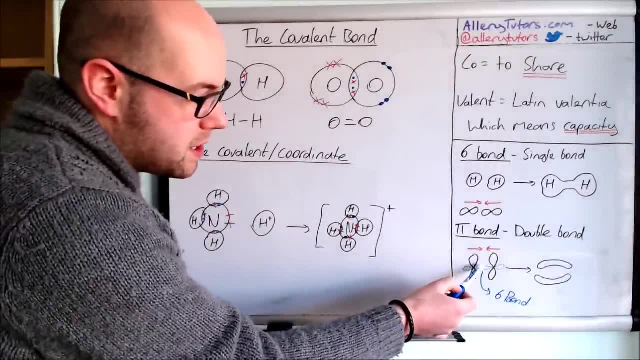 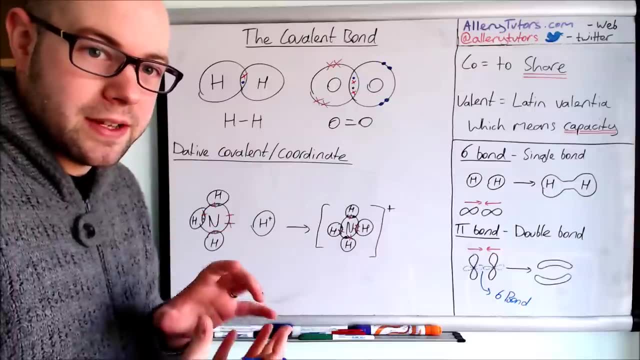 And you have both of them there. So you have the sigma bond in the middle and you will have the pi bond. So this is effectively makes up the double bond. It's the sigma and the pi put together. So this is the double bond. 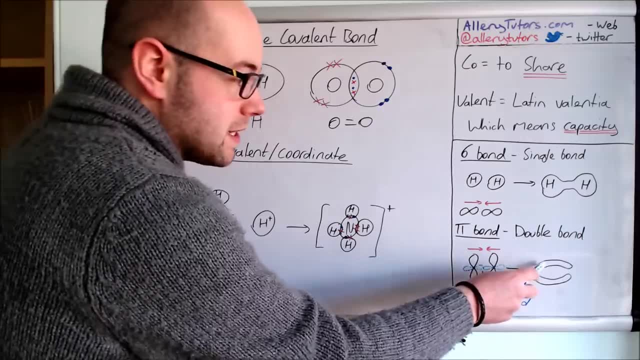 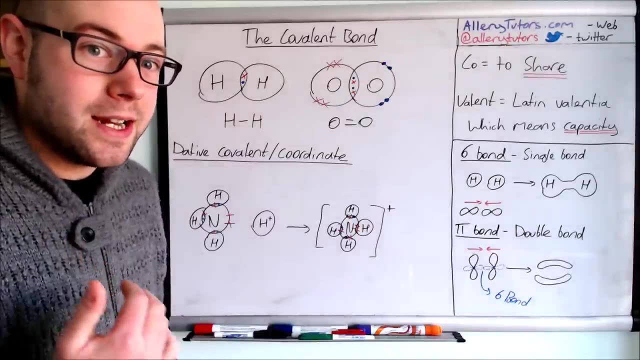 Now, something a little bit weird about this is these, this actual blobby bits here. This shows you where the electron will be, or where an electron could be At any one time. This is like a probability. It's like a. it's not actually. the electron doesn't follow the outside of the actual orbital. 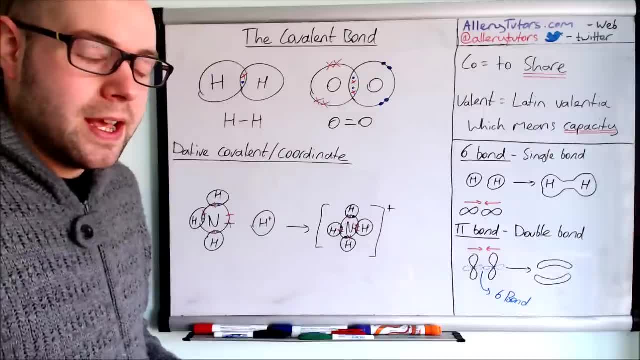 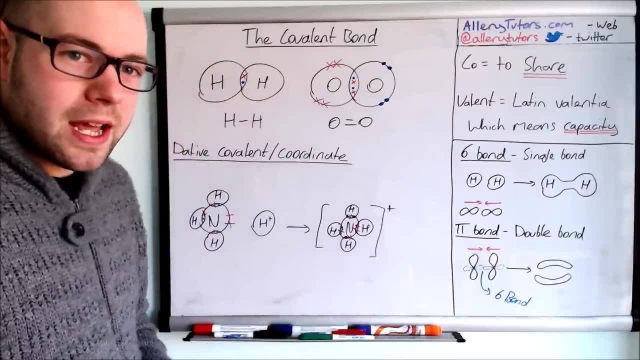 It just. this is like a map of where the electron could be at any one time. Now you'll notice that actually, if you look in the middle, there's no chance of the electron being there at all. This is in the middle here because there is no space in the middle. 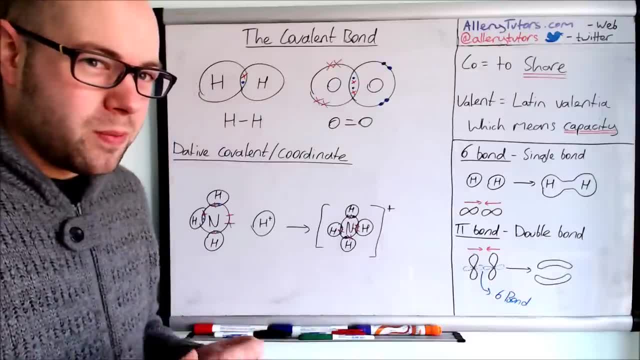 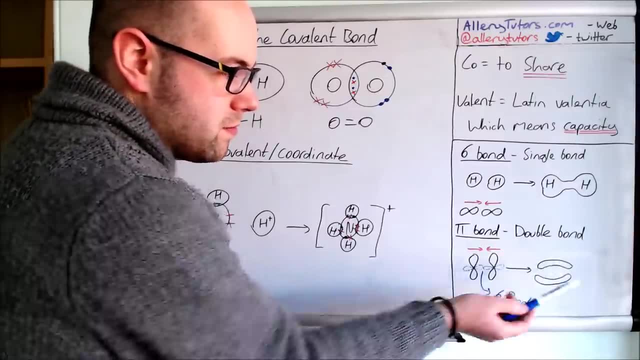 It's nipped in right at the middle like an hourglass. So this is a bit weird because actually in an electron, in a pi bond, we have an electron here, An electron In here, But actually sometimes the electron. you don't have to have one electron in the bottom or the electron at the top. 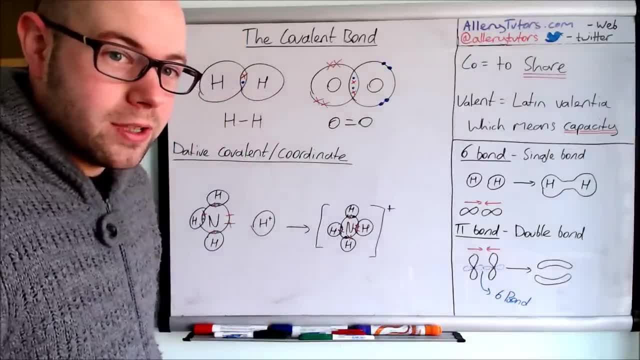 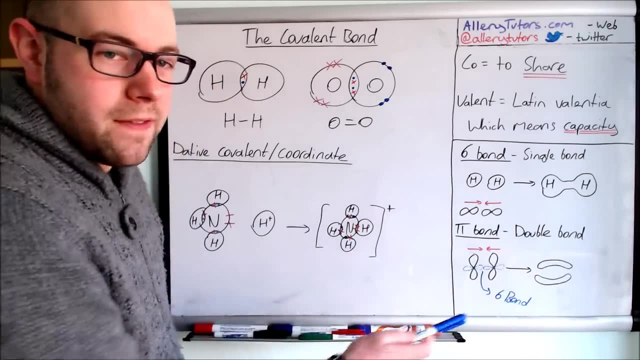 It could exist anywhere in them. two orbitals. Now this is a weird question for you maybe to think about. is that how does an electron get from this lobe to this lobe if there's no possibility of them being in between? So that's a little bit weird. 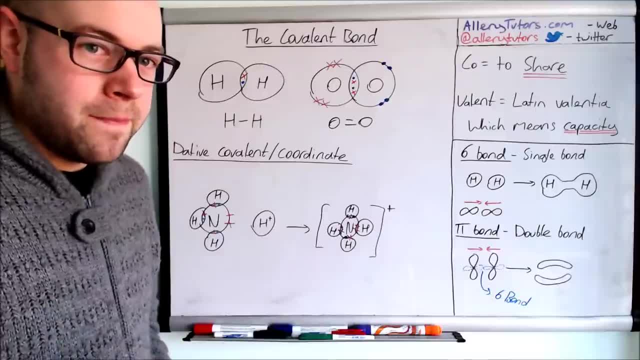 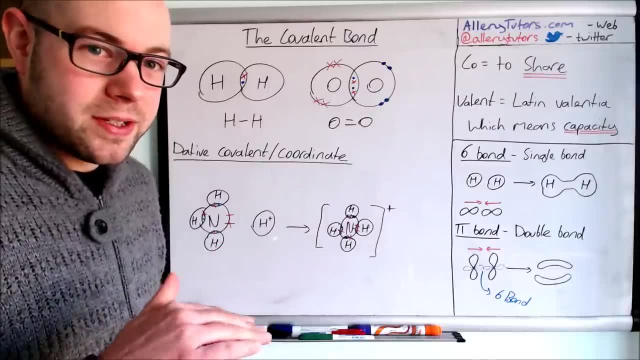 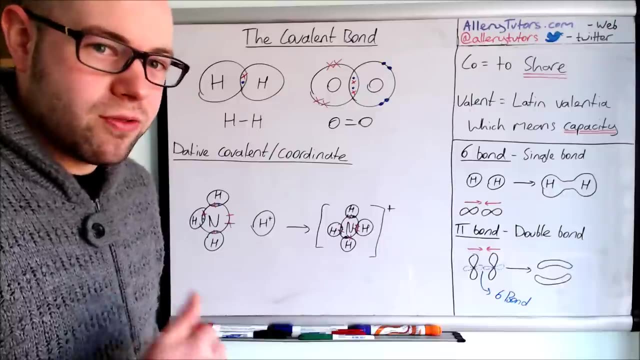 And it actually throws into doubt whether an electron is actually a particle, And in fact, if we look as electron as a particle, it can't be, It can't be explained, It's impossible to explain it. So we have this kind of like a wave theory, or we call it a wave principle of electrons, and something that Schrodinger tried to look at as well. 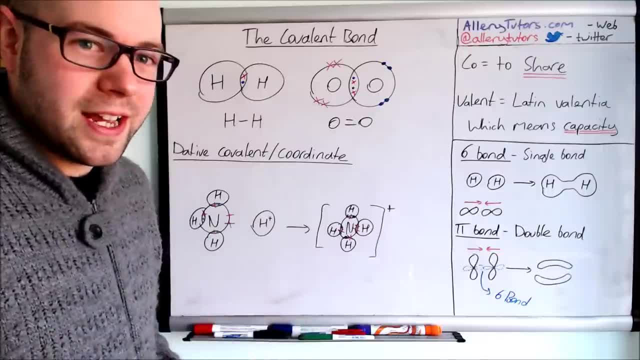 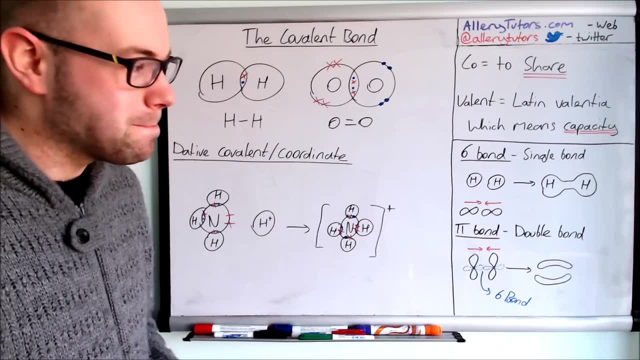 So if you're interested and you want to look at that further- thankfully this is not in the A-level syllabus, But if you're interested in that, just have a look at Schrodinger's equation. You'll see perhaps how complicated this could be. 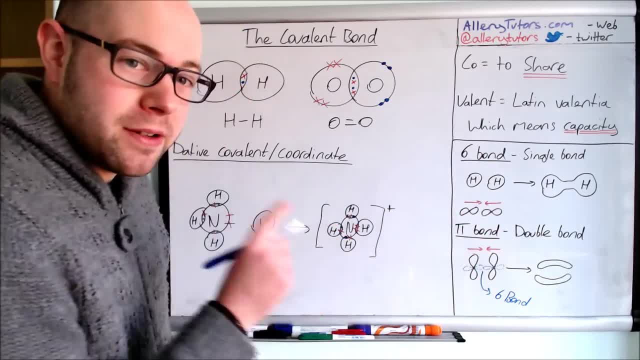 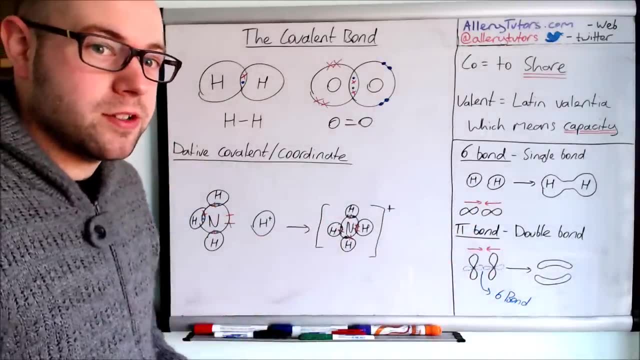 But yeah, as long as you understand about the sigma and the pi. I know some exam boards know They do want you to know how A pi bond and a sigma bond works. You need to check your specification to make sure you know this. 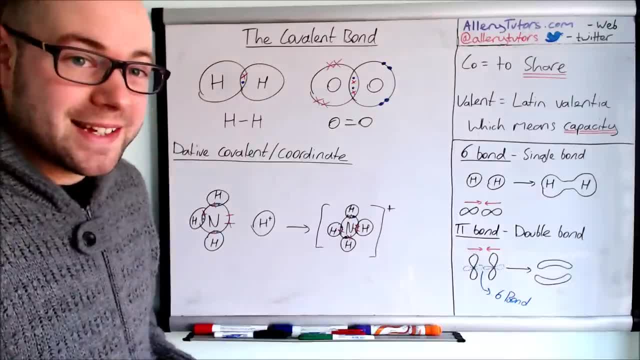 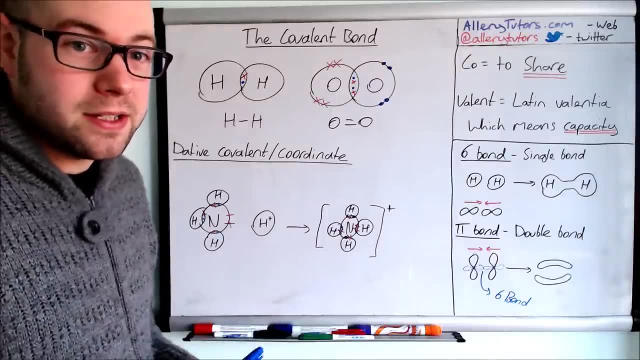 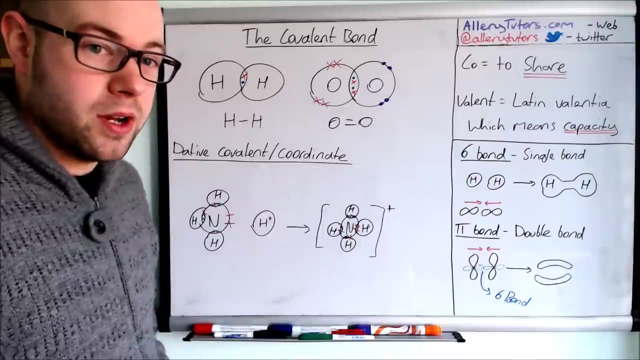 Some exam boards literally just want you to know: sigma bond is single, Pi bond is double, particularly in topics like alkenes and bonding. So check the specification, the alkenes topic for pi bonds in particular and bonding, And if it doesn't require you to know how these things work, then you should be OK. 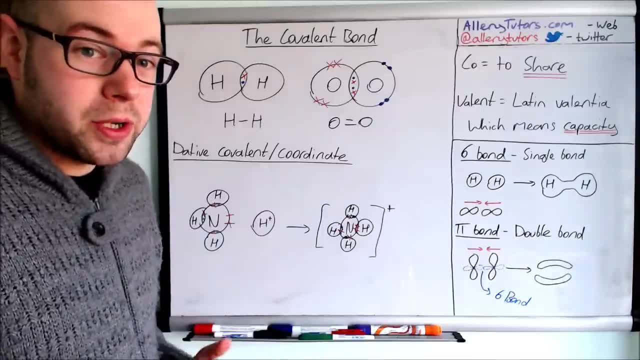 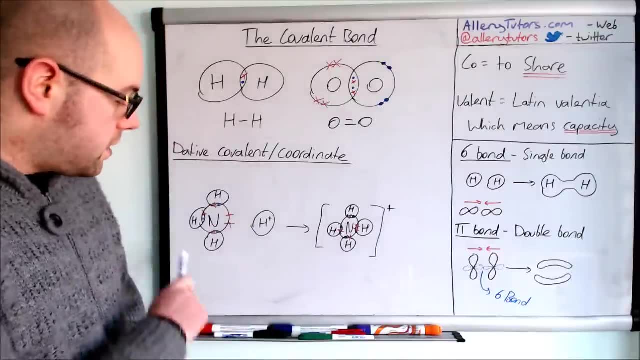 And the final thing is dative, covalent or coordinate bonding. So you can see here this is a slightly different type of bonding. It's weaker than a traditional covalent bond And you can see we've got ammonia here. Ammonia has five nitrogen has five electrons. 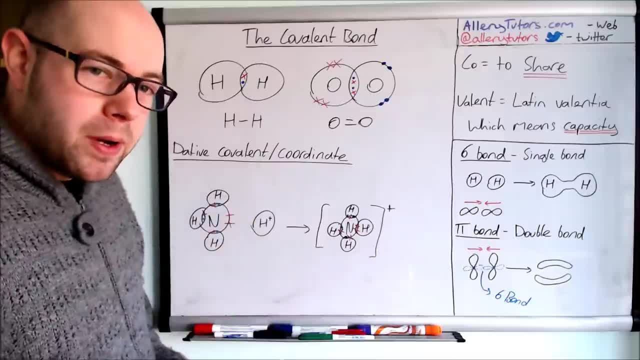 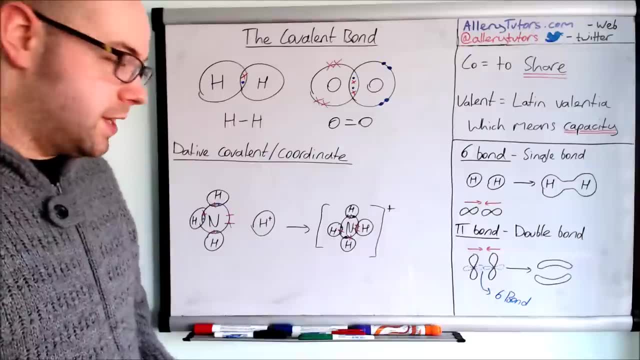 And it's got three hydrogen surrounding it, And a dative covalent bond is basically where both pair of electrons are donated from one atom to another atom or ion, And in this case we're going to react ammonia with a H plus ion, which is over here on the right. 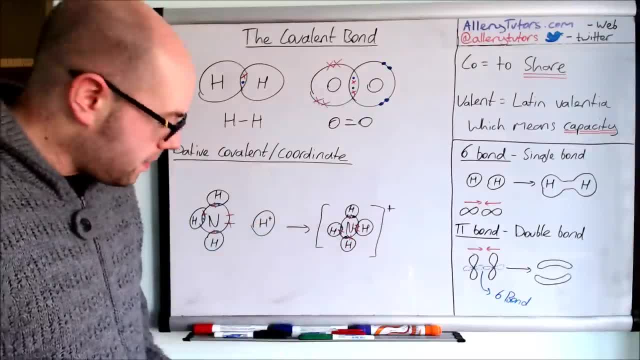 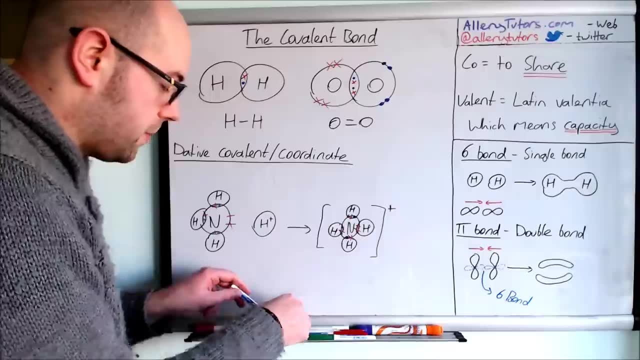 And we're going to form an ammonium molecule. Now you can see I'm going to draw this as a displayed formula to show you how it works. We've got the dot cross already there on the board, So the displayed formula we're going to put here. 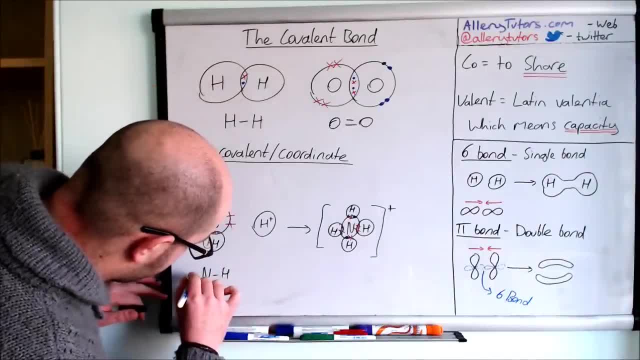 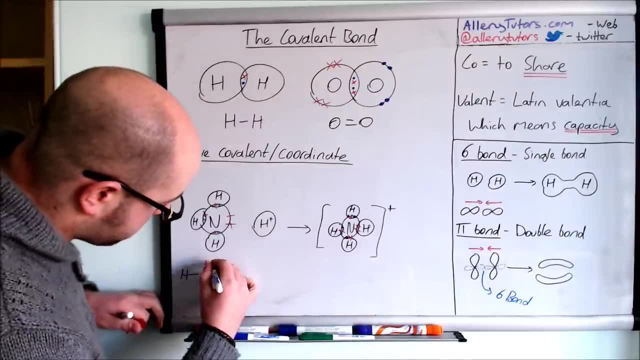 So this is NH3 and this is ammonia. Now ammonia has that lone pair of electrons on the nitrogen And that's crucial For a dative covalent bond. you must have a lone pair of electrons And we're going to react that obviously with your H plus. 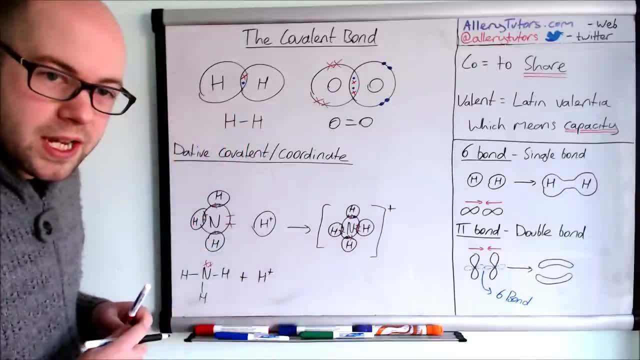 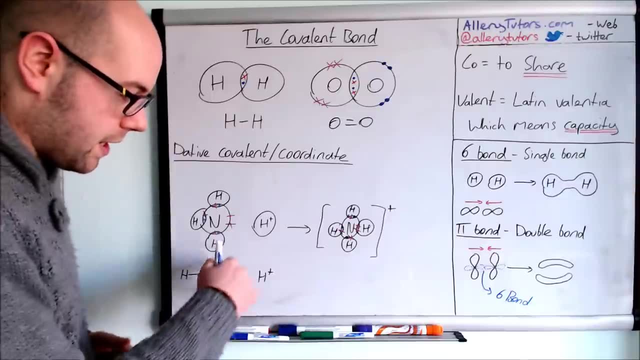 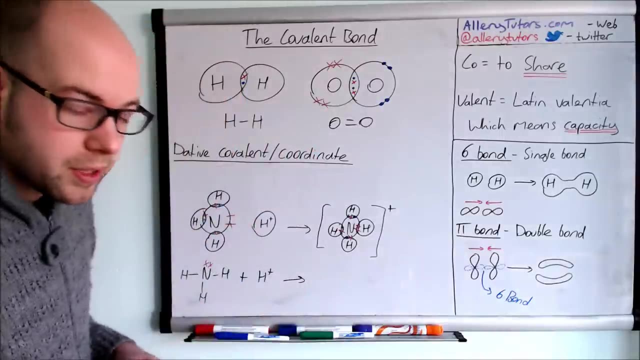 So it's literally: there is no bond here, It's just H plus This is a hydrogen ion. It's basically a hydrogen atom without an electron attached to it. So it's just a proton. effectively, That's what's left, And then we're going to form, obviously, our dative covalent bond. 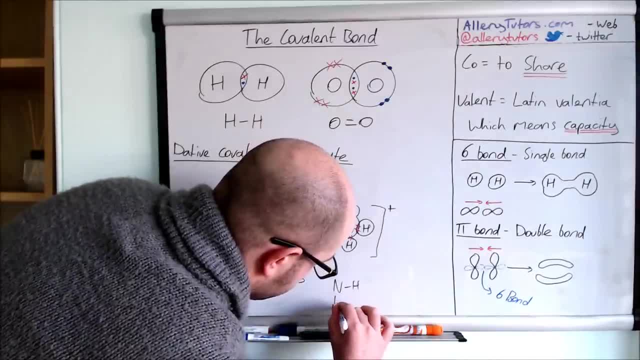 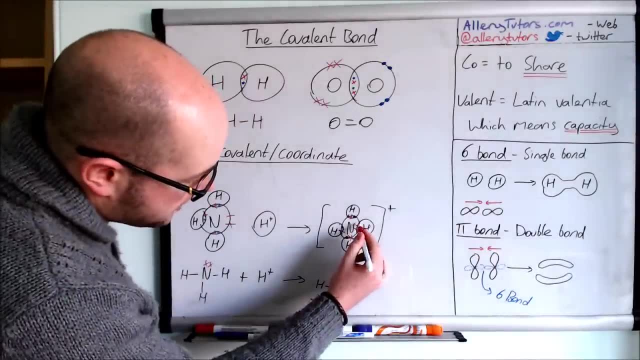 So this is nitrogen hydrogen, hydrogen hydrogen, Right Now the dative covalent bond, if we have the lone pair of electrons on the nitrogen. so you can see there, see that Two electrons And these are donated. 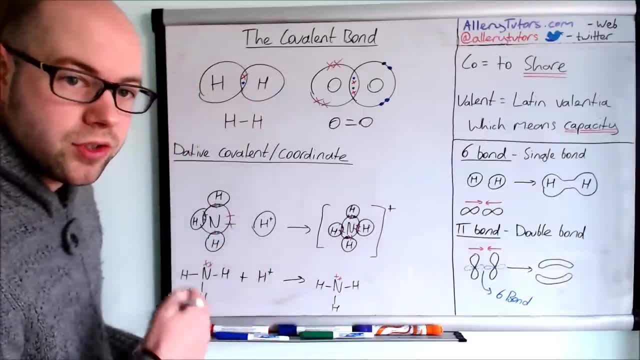 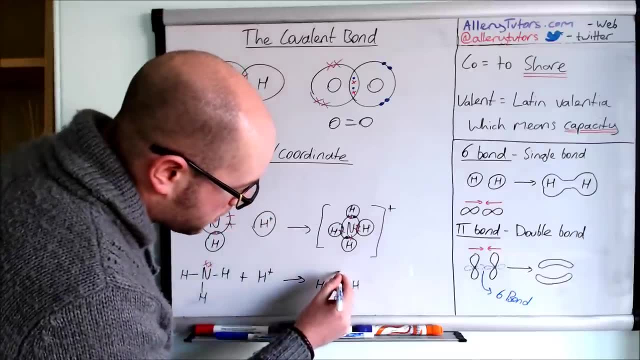 Both of them are donated to the hydrogen. It doesn't have any electrons to share, So it can't form a normal covalent bond. It doesn't have any electrons, So we're going to draw a dative covalent bond or coordinate bond. 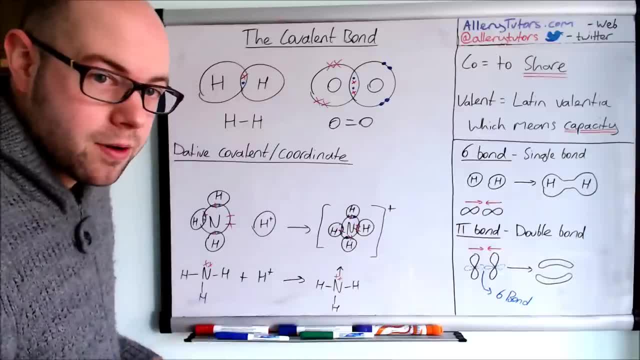 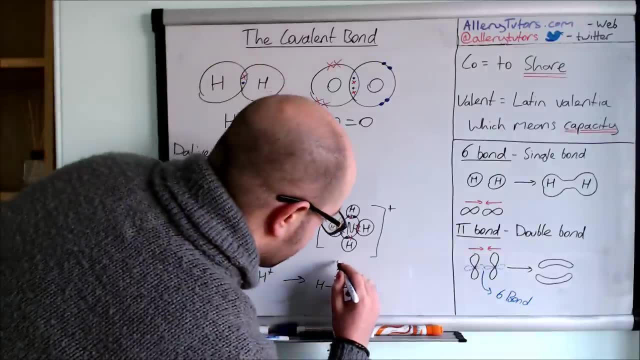 And this is unique because it's actually now represented as an arrow, And the arrow always shows where the electrons are going from and where they're going to. So make sure you draw that correctly in the exam as well. Stick the hydrogen on And then we draw a square bracket around. 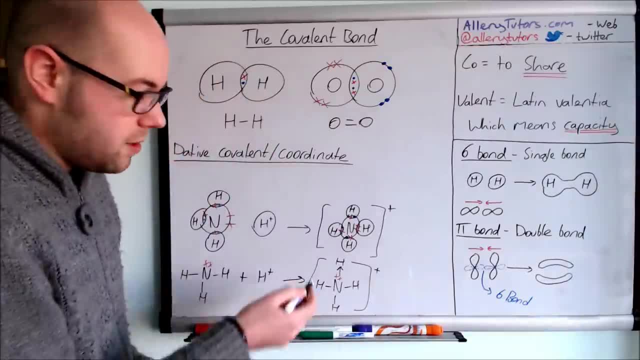 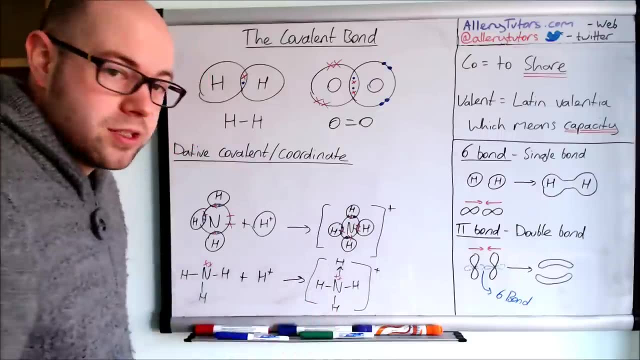 And positive charge. The whole thing now has a positive charge Because we've effectively added the H plus sign onto the end there. So we put the plus on there, But make sure you draw it as an arrow. That's the dative covalent bond or the coordinate bond.